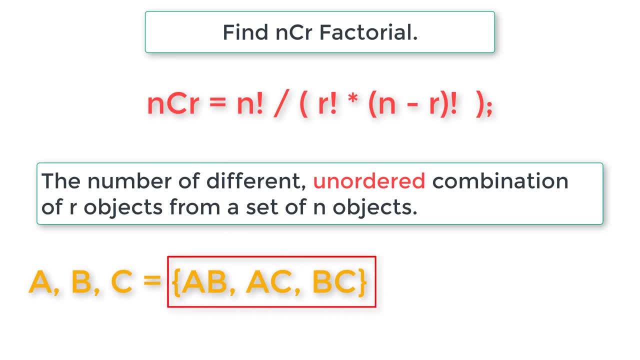 of r. So this entire set is the result. that is, we have three objects inside this set. So 3c2, that is 3, is n value. r value is 2.. So the result, ncr, will be 3.. So let's. 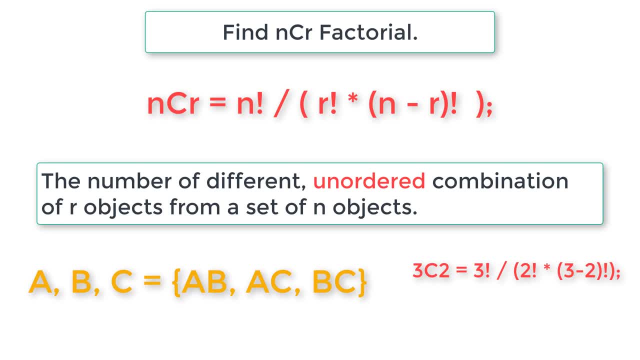 calculate. Calculate that using the formula: So 3 factorial is 3 into 2 into 1.. 2 factorial is 2.. 3 minus 1 is 1 factorial. So 3 into 2 is 6.. So now 6 division 2 is 3.. So 3c2, that is factorial. 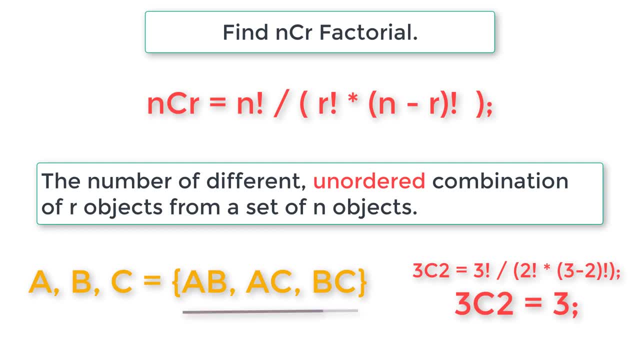 of n and r. that is 3 and 2 is 3.. So also an important note here: n should always be greater than r, because we can fetch 2 out of 3, but we can't get 3 out of 2, right? So n should always be greater than r. So this: 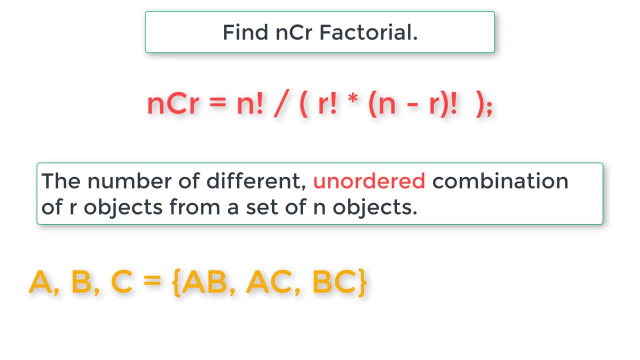 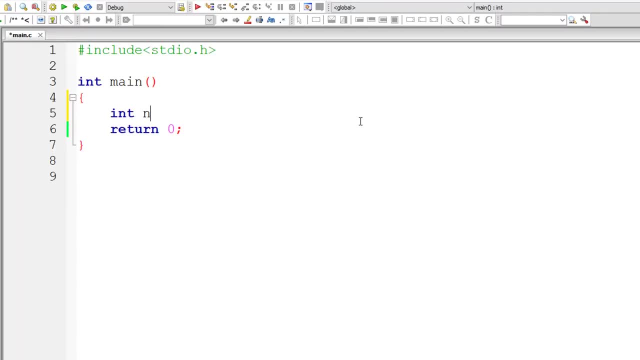 is very important, So hope you understood something in this. These details are not required for you If you know the formula. that's enough for now for computer science students Going forward. you need to understand why you are writing this code, why you are using these. 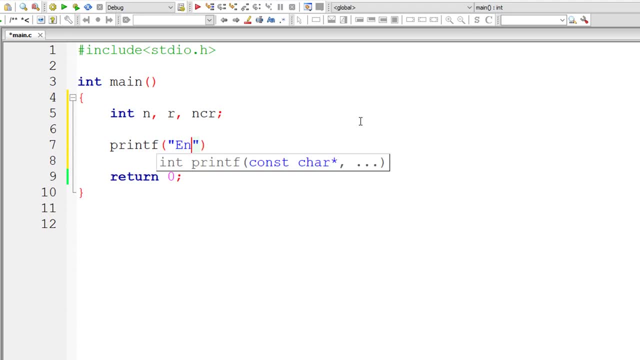 formulas. That's very important, okay, So for now let's write the c program. I'll take three integer variables, nr and ncr. I'll ask the user to enter a positive value for n and r. So let me store that inside the address. 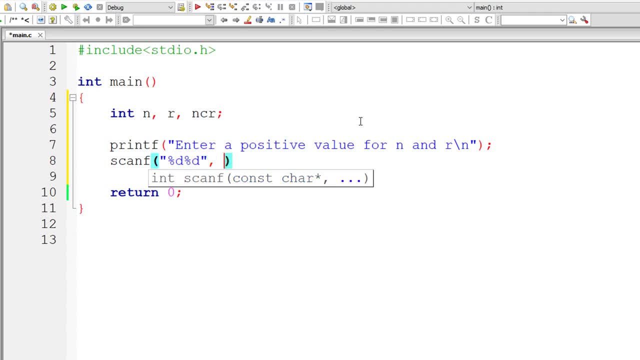 of integer variables n and r. So I'll write the formula here: ncr is equal to n factorial division, r factorial into ncr. Okay, Okay, Alright, minus r factorial. so this is what we saw it in our previous screen, right? so we need to write this: 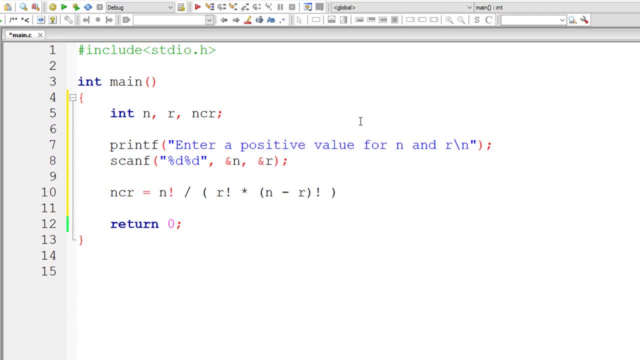 using c programs, arithmetic operation roots. so let's do that. ncr is equal to. i'll write a function called factorial, so factorial of n. this would return factorial of n division. let me copy this division: r factorial multiplied with factorial of n minus r. so that's the formula. 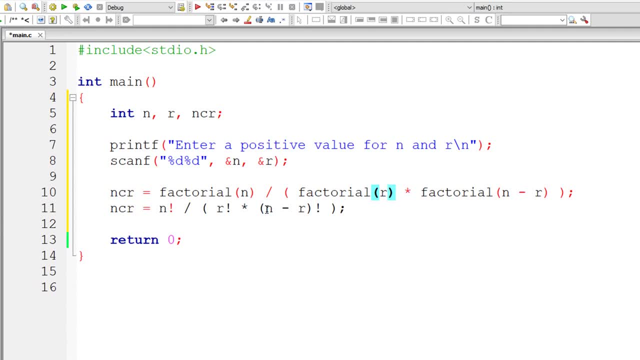 n factorial, r factorial, n minus r factorial. so let me remove this. let me write printf statement here. printf ncr. factorial of percentage d and percentage d is percentage d. so the first percentage d is that of n, variable n, the second percentage d is that of r and the last percentage d 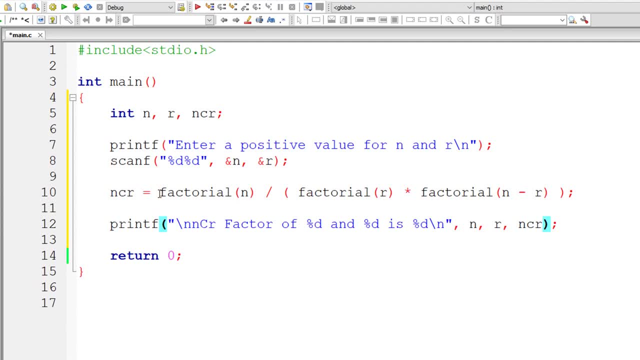 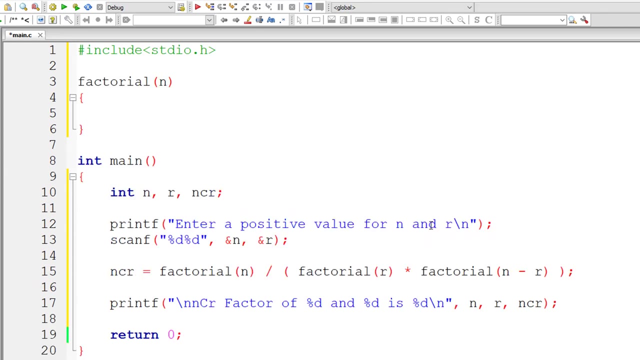 is that of ncr, the variable ncr, so we need to define factorial function. now, all these take only single parameter, single argument. also, note that we have division operator in this formula, right, so you may get floating point values. in this case you will be getting integer value, but 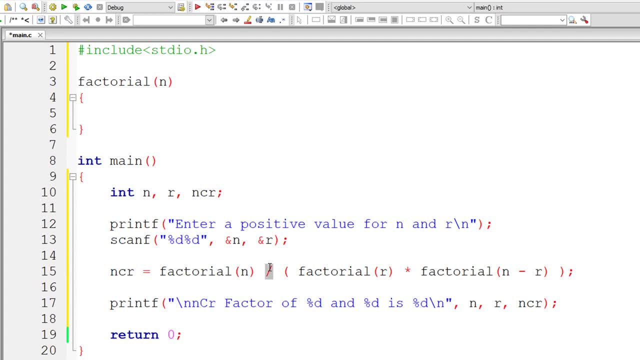 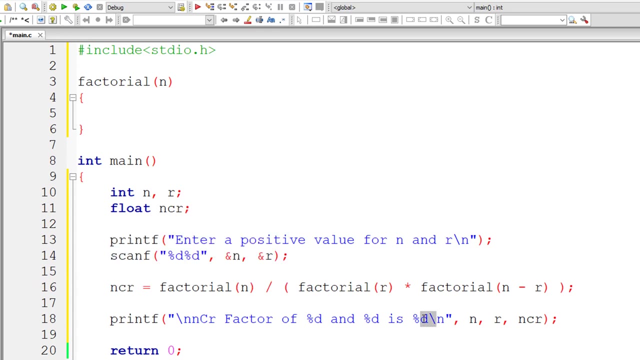 whenever you there is formula and involvement of division, it's always better to have floating point variables. just make sure to have floating point variables for accuracy. in this case it's it may not hold good, but practice this. it's best practice to declare it as floating point. 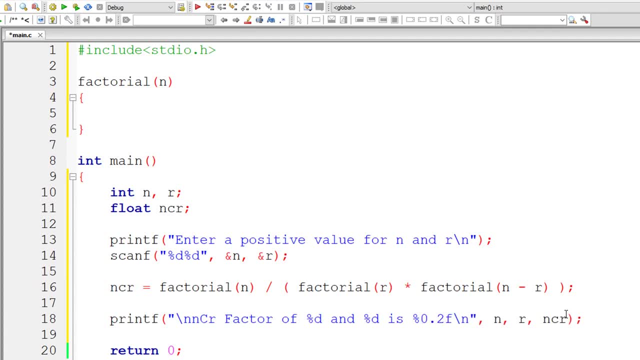 values. so i'll write 0.2f. but factorial returns integer value, not float, okay, don't get confused here. factorial returns integer values, okay, division of which might result in floating point results. so I am taking ncr as floating point value. factorial still returns integer type value, okay. 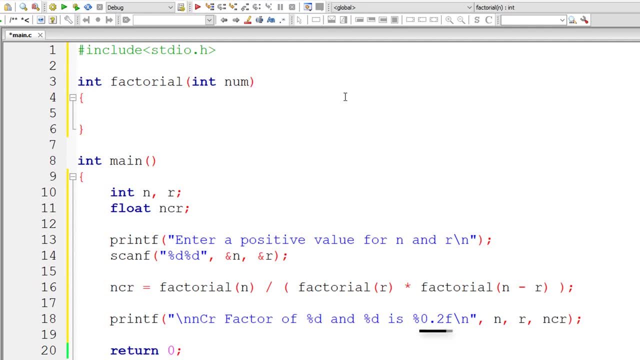 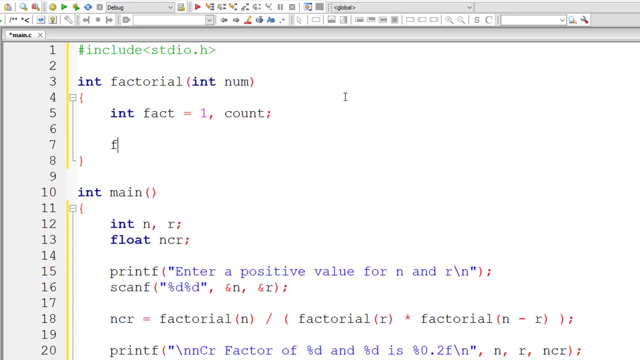 so we are using format specifier percentage f. okay, so I'll take a integer variable fact and assign one to it. I'll take another variable, count for loop, counter variable, for I'll initialize count to one and iterate through this for loop until count is less than or equal to user entered. 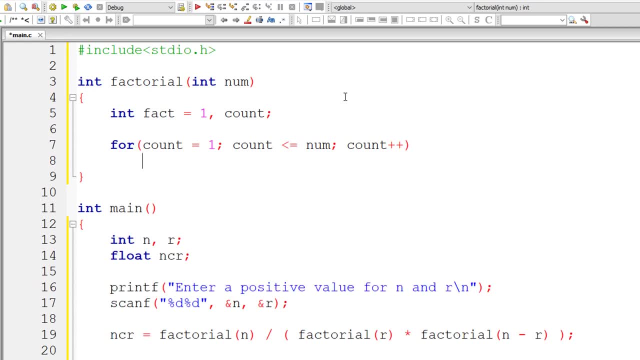 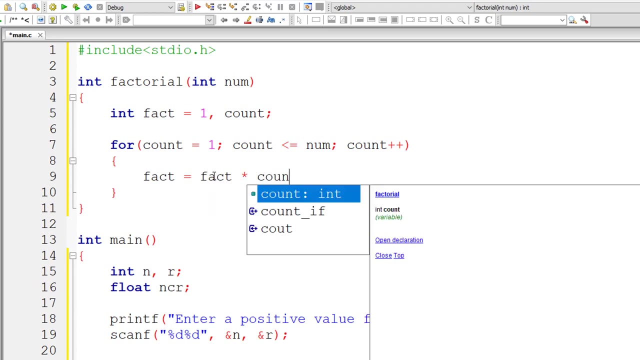 number. and for each iteration of this for loop, I will increment the value of count by one. so here I'll write fact. I'll tell you why I've assigned it to one. so before that, let me write the logic- fact is equal to previous value of fact- into the value of count. let me even return the value of. 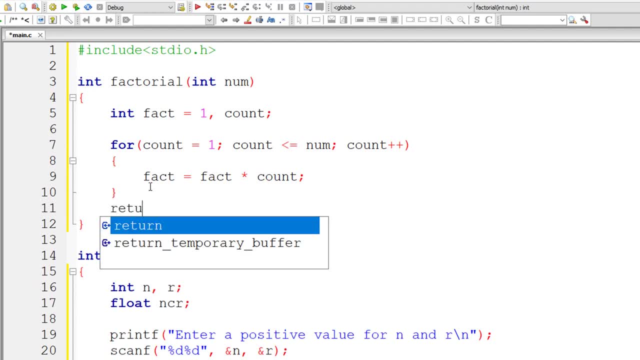 outside this for loop return the value of fact. so if fact value is actually 0, we have multiplication here. so 0 into anything will always be 0, so fact will ultimately be 0, which will be wrong. so 1 into any number will be that number itself. it don't affect. 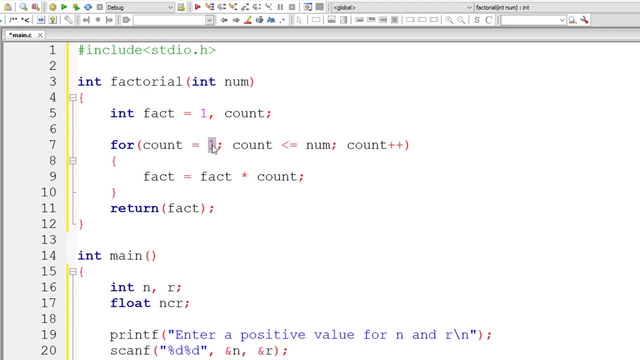 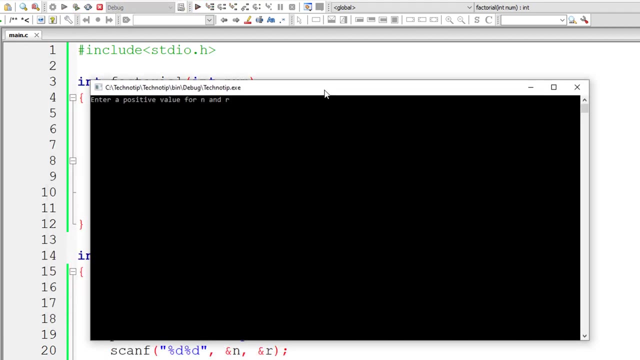 the multiplication. so it starts from 0. sorry, it starts from 1. so complete logic for finding factorial is present in the link present in the description section of this youtube video and also i'm showing it on your computer screen. please visit it to get the complete logic. i'll enter 3. 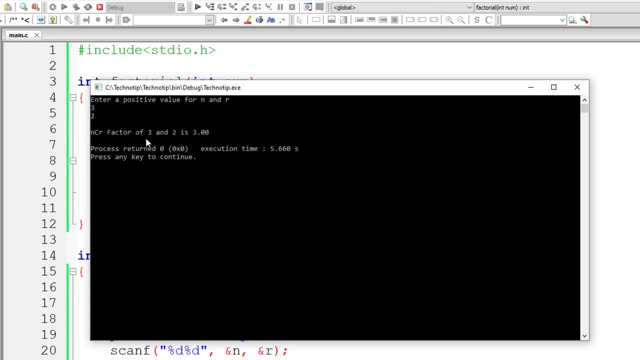 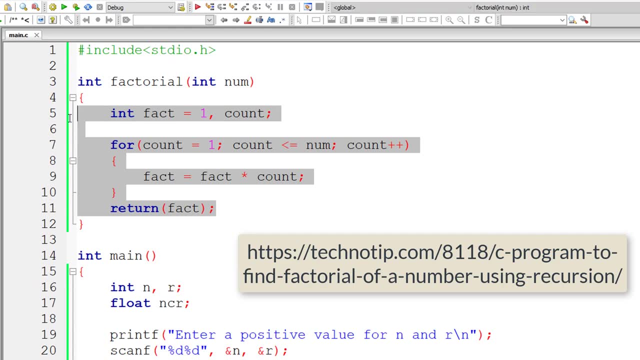 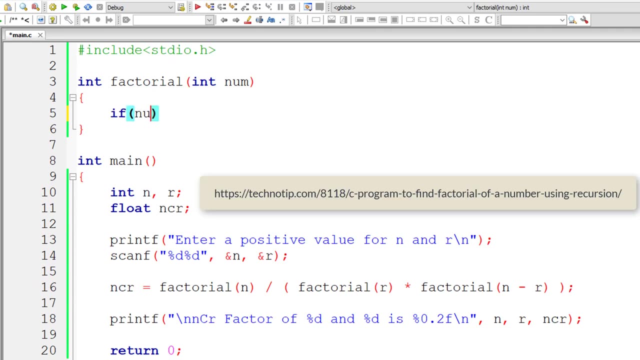 for n and 2 for r. so ncr factor of 3 and 2 is 3. we saw that in our example, so let us do the same thing using recursion. i have explained the recursion logic to find factorial in a separate video link to which i am showing you on your computer screen. please follow that. 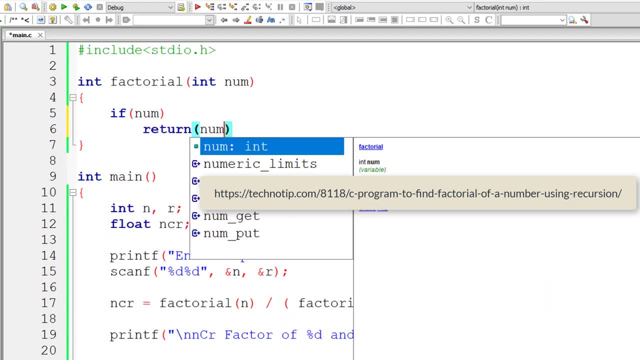 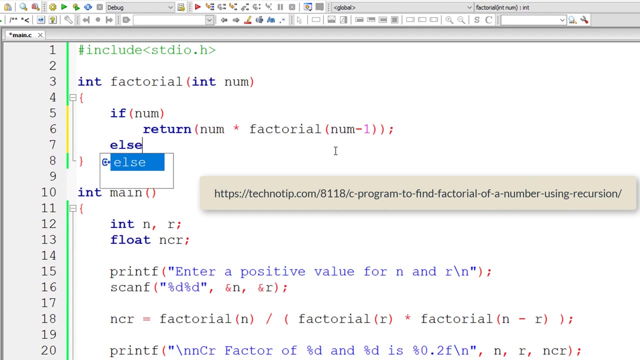 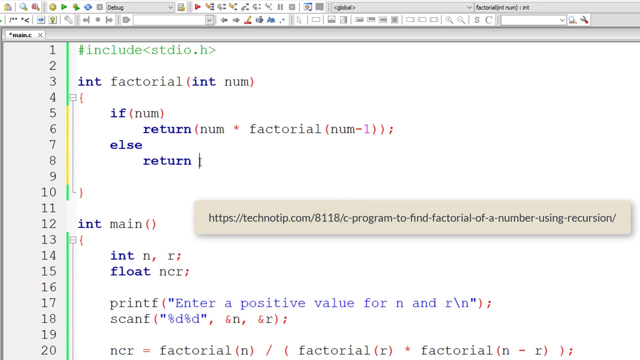 and watch that video. so if num is non-zero, then num into factorial of this is recursive call factorial of num minus 1. okay, let me write base condition in else part. so if num is 0, then 0, factorial is 1, so let us return 1. so that's it. this should work too. 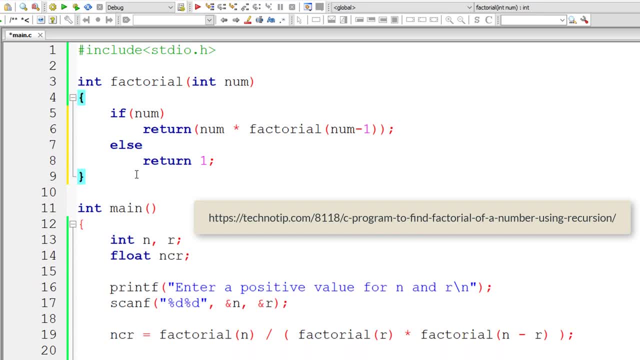 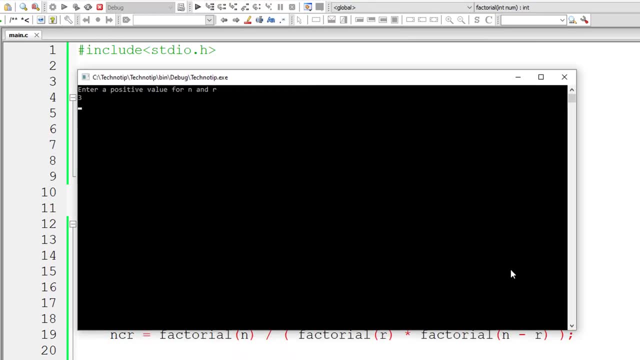 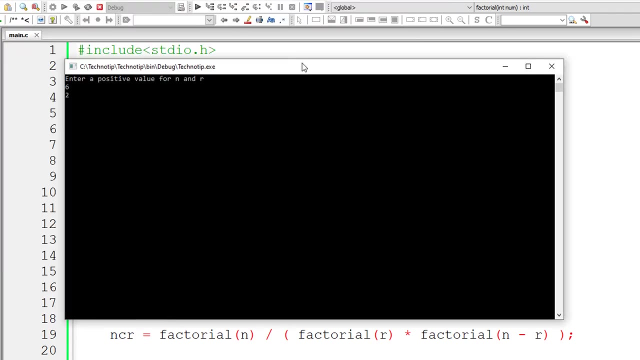 so please visit the link present in the description section of this video and description section of this youtube video to know the complete logic about the working of this factorial function. we have a separate video for that. so far, ncr factorial is 3 again, so 6 and 2. 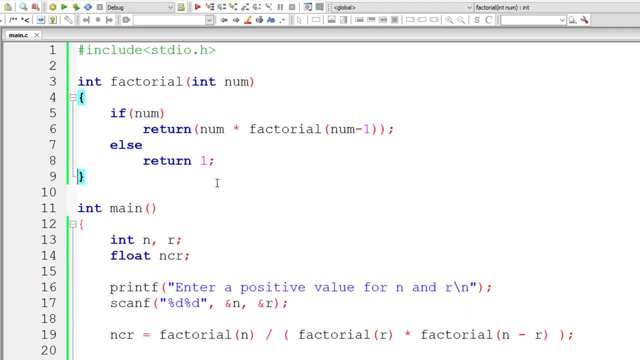 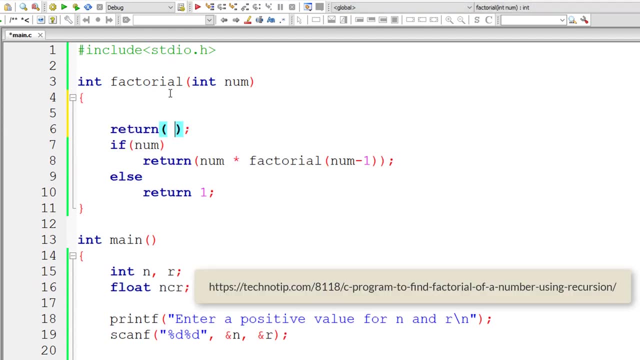 the ncr factorial is 15. so now let me write this in single line of code, using ternary operator return. so i have explained even that, the complete logic, so link to, which is present in the description section of this youtube video again. so, when this number is not equal to 0, then return this.